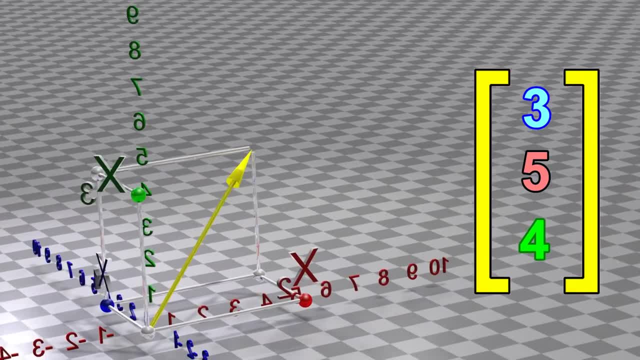 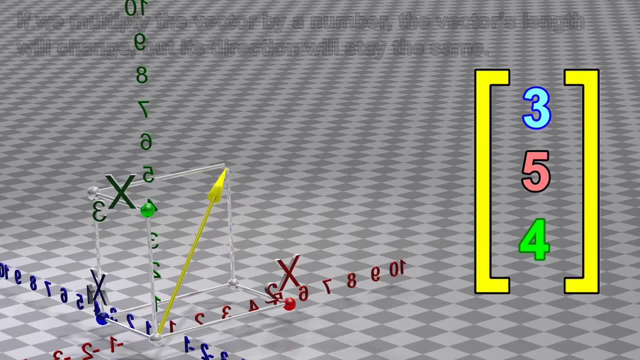 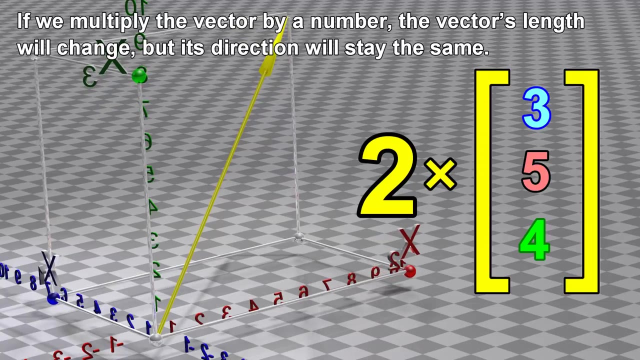 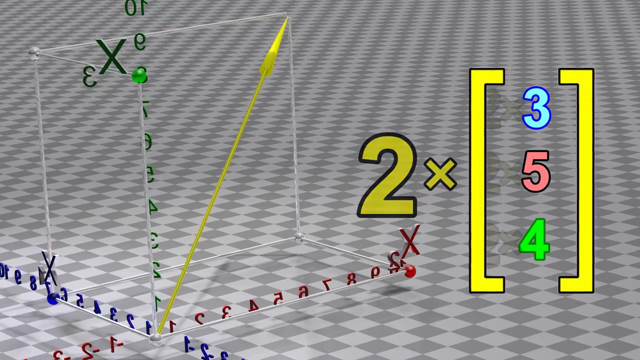 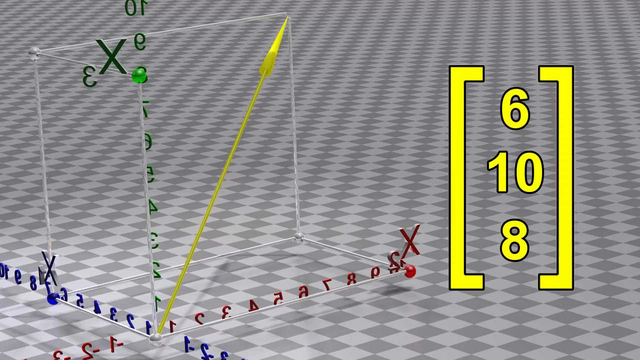 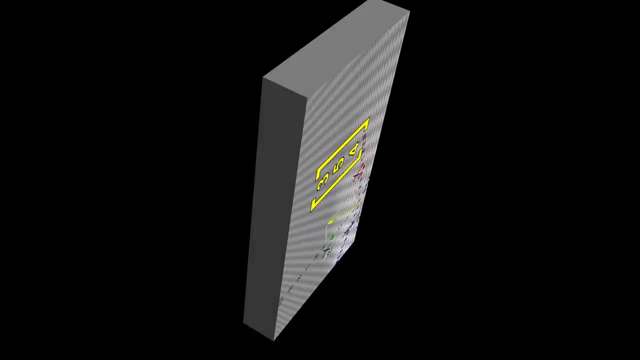 Each vector has a length and a direction. If we multiply the vector by a number, the vector's length will change, but its direction will stay the same. So each quarter will be an arrow and each bullet will be a tipofa. 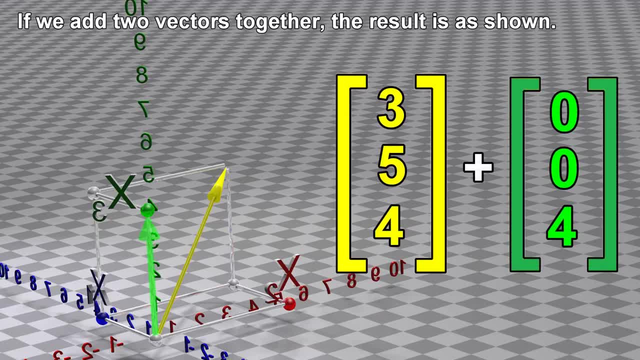 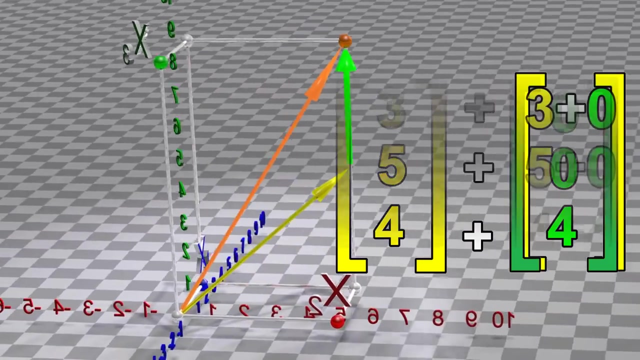 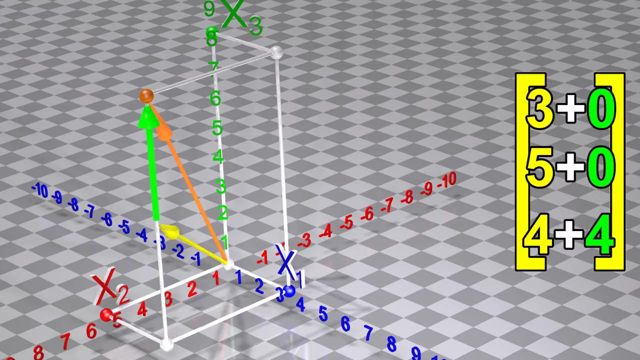 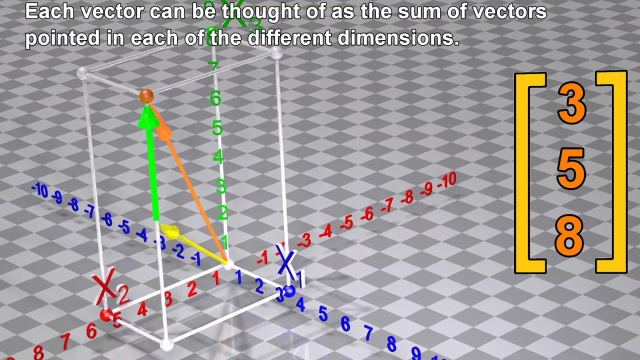 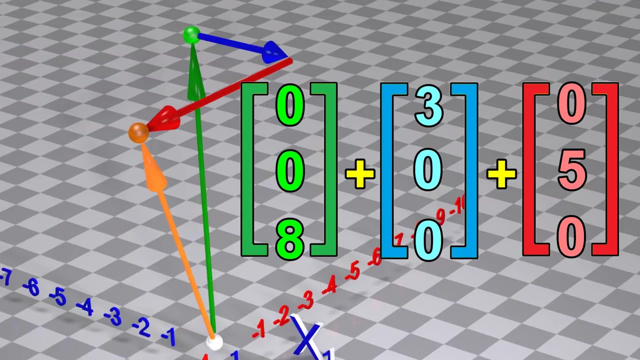 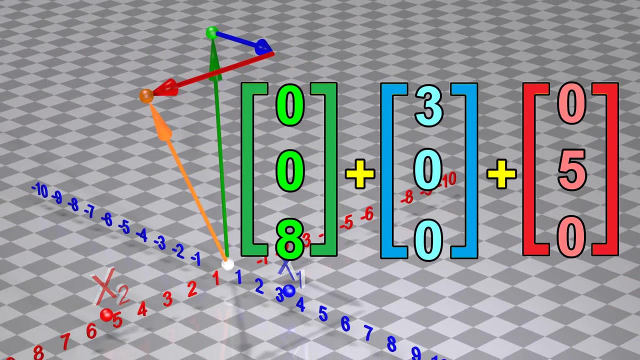 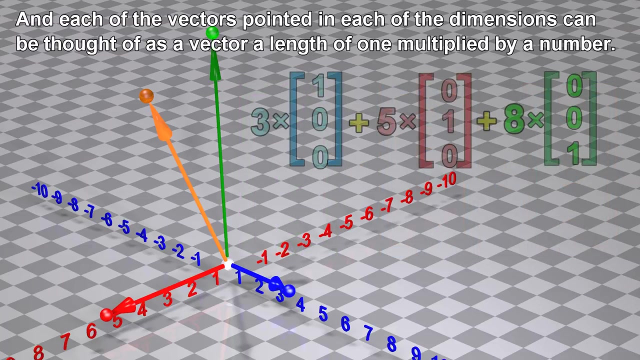 If we add two vectors together, the result is as shown. Each vector can be thought of as the sum of vectors pointed in each of the different dimensions, And each of the vectors pointed in each of the dimensions can be thought of as a vector a length of 1 multiplied by a number. 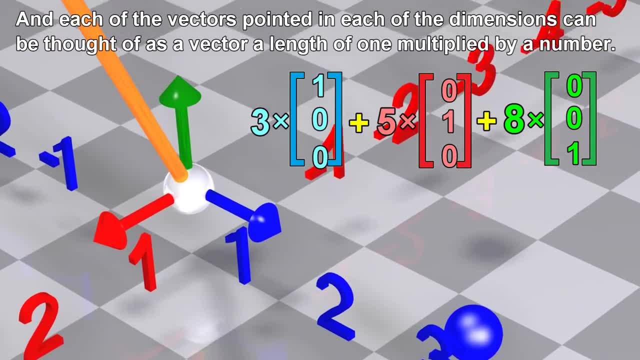 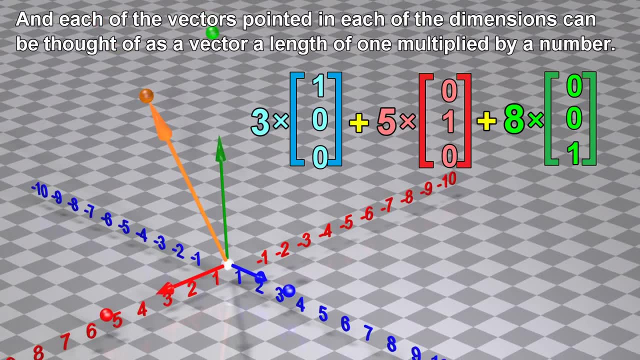 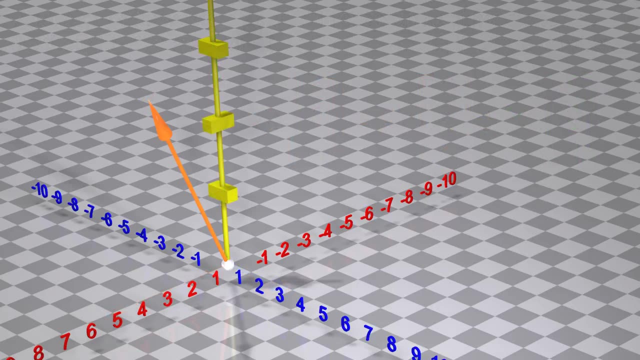 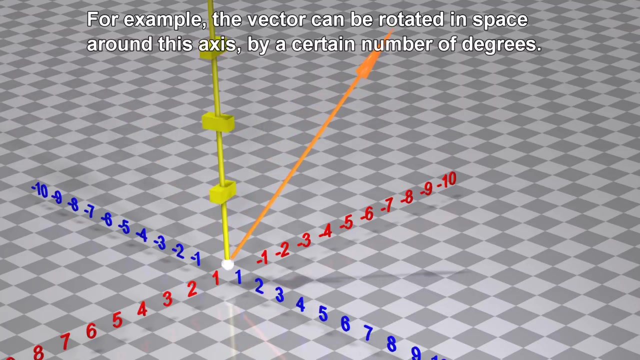 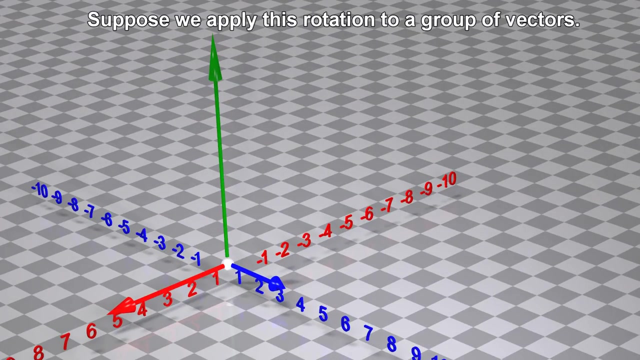 There are many transformations that can be applied to a vector. For example, the vector can be rotated in space. The vector can be rotated in space around this axis by a certain number of degrees. Suppose we apply this rotation to a group of vectors. 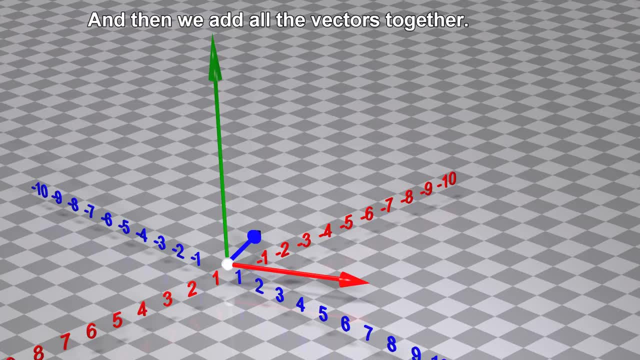 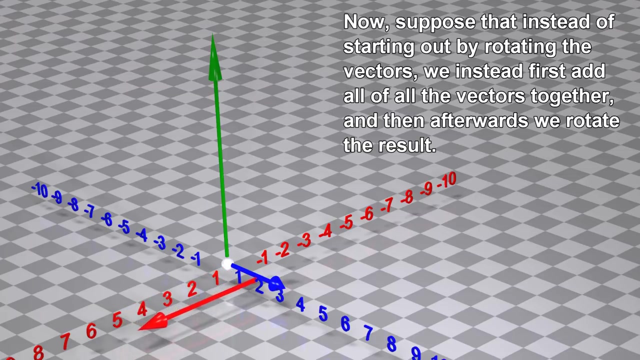 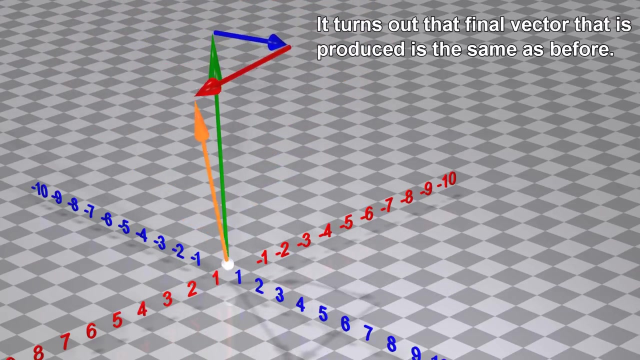 And then we add all the vectors together. Now suppose that instead of starting out by rotating the vectors, we instead first add all of the vectors together and then afterwards, we rotate the result. It turns out that the final vector that is produced is the same as before. 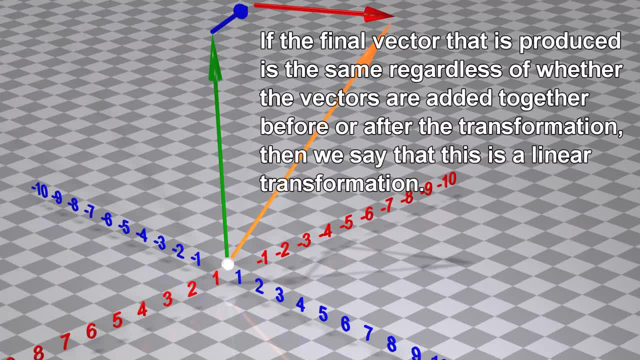 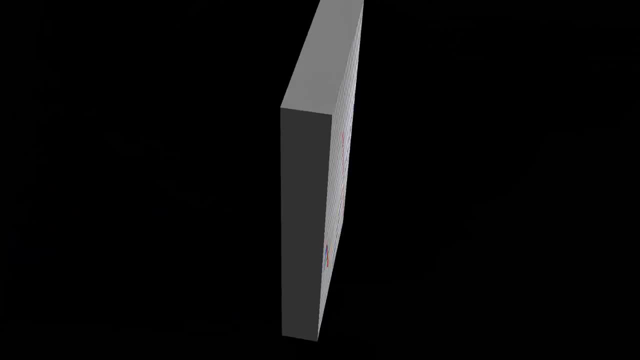 If the final vector that is produced is the same, regardless of whether the vectors are added together before or after the transformation, then we say that this is a linear transformation. Another example of a linear transformation is that the vector is stretched or squeezed, as shown. 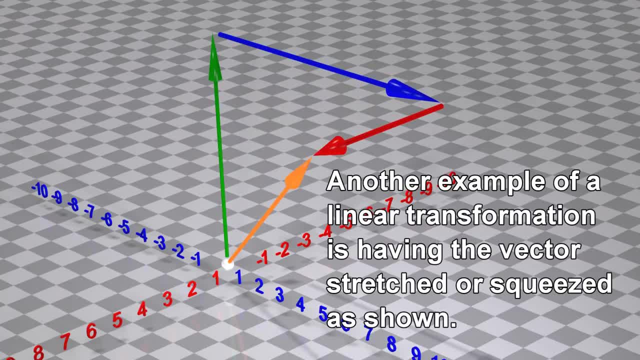 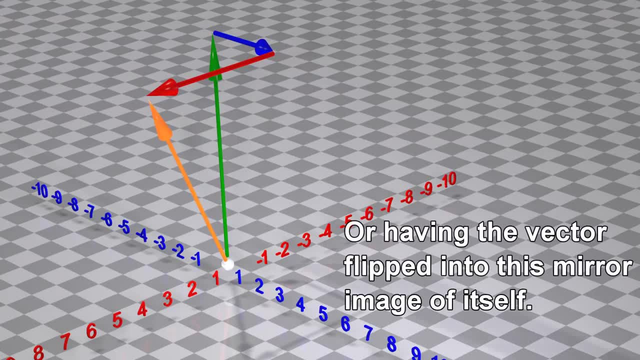 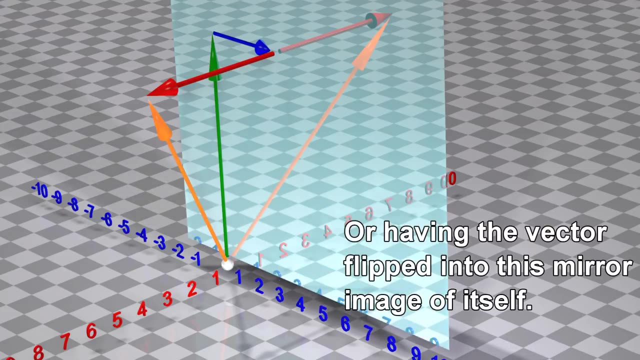 If the vector is stretched or squeezed, it is like a moving object. Or if the vector is flipped into the mirror, it becomes like a moving object, And that's all you need to know about where a vector is. Another example of linear transformation is having the vector stretched or squeezed, as shown. 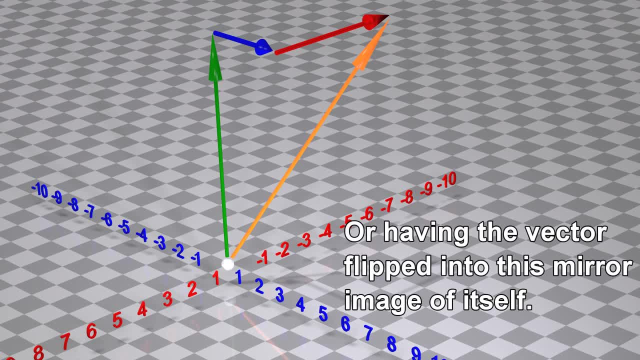 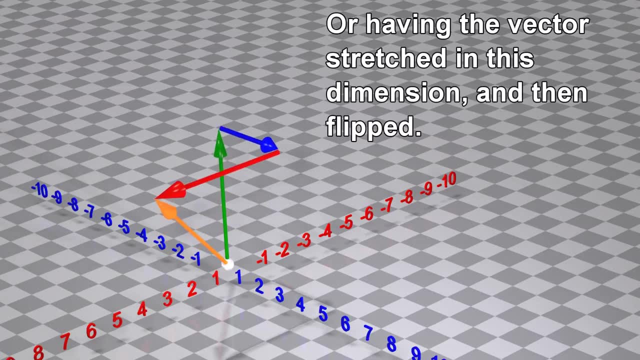 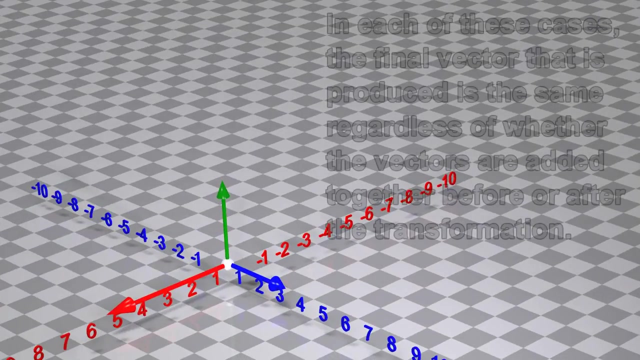 Or having the vector flipped into this mirror image of itself- For more information, visit Huxleycom- or having the vectors stretched in this dimension and then flipped. In each of these cases, the final vector that is produced is the same. 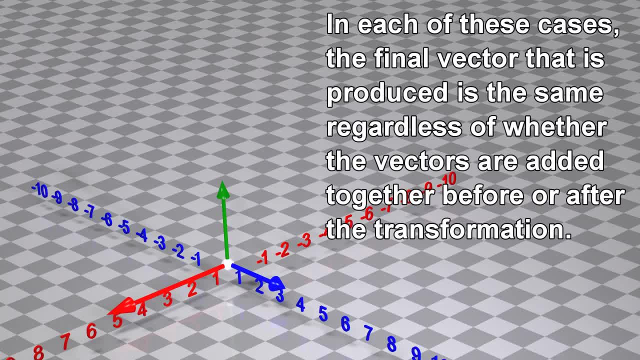 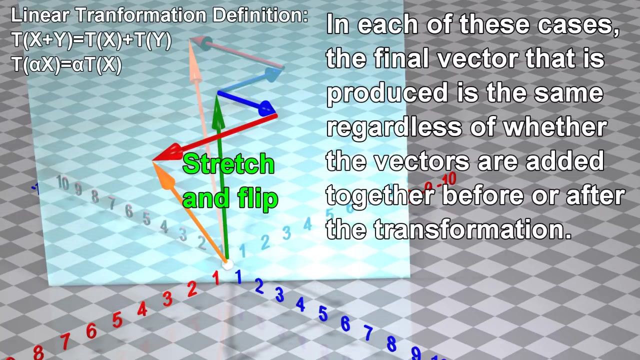 regardless of whether the vectors are added together before or after the transformation. In each of these cases, the final vector that is produced is the same, regardless of whether the vectors are added together before or after the transformation. This is the definition of a linear transformation. 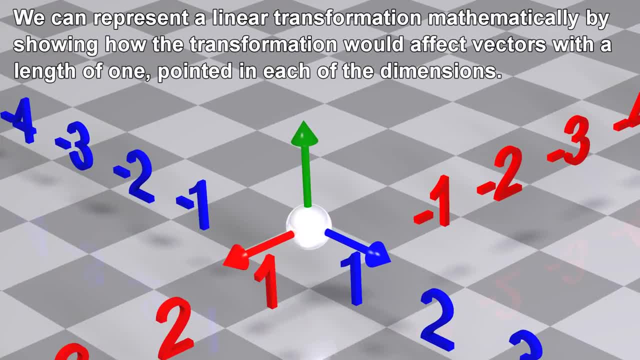 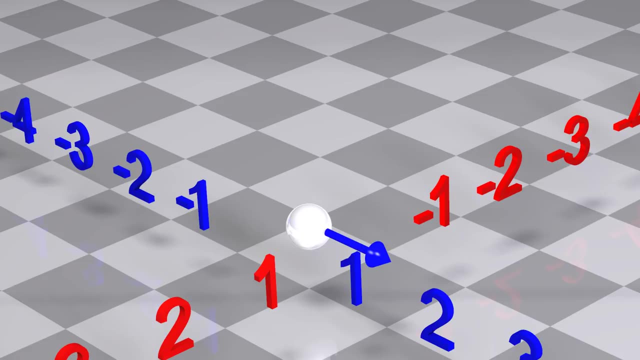 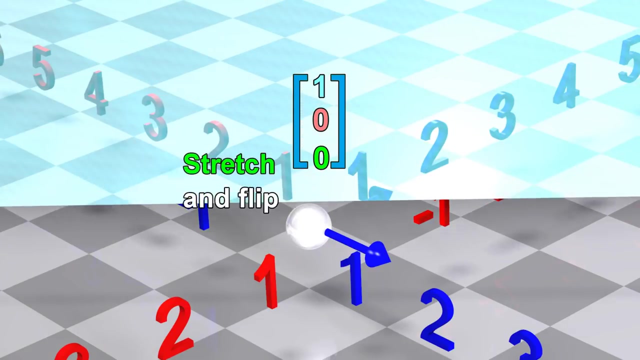 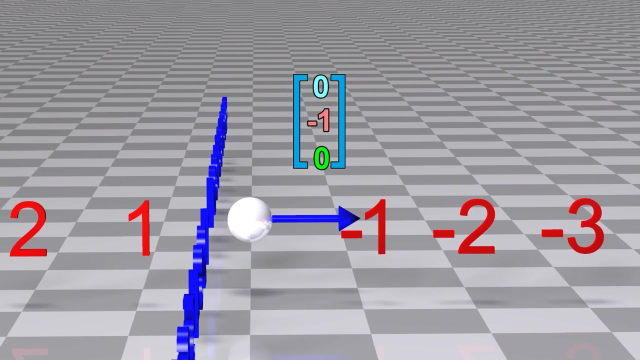 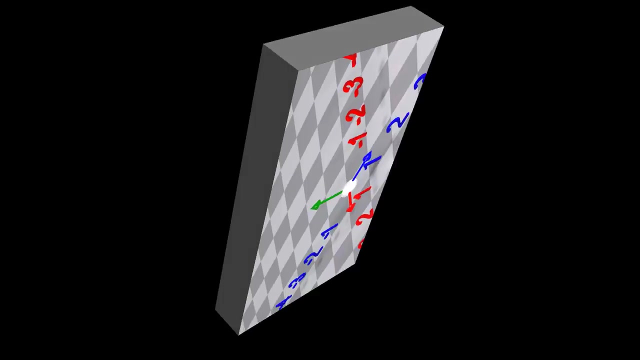 We can represent a linear transformation mathematically by showing how the transformation would affect vectors with a length of 1, pointed in each of the dimensions. We can also show how a vector of X-shape would be evaluated. In this diagram we can see that there are two vectors that will be evaluated. 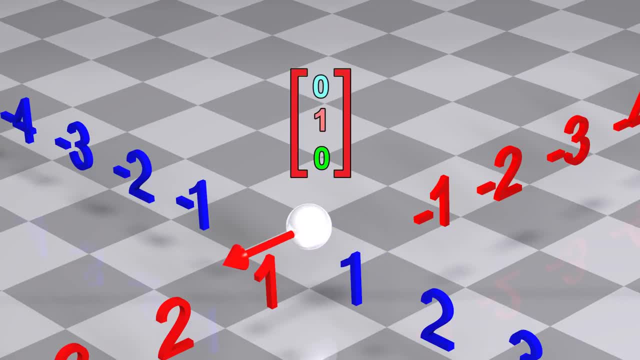 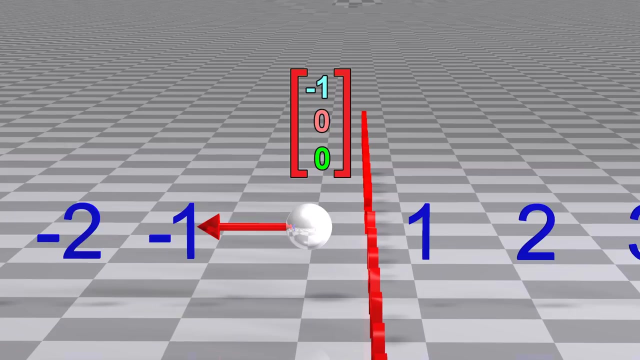 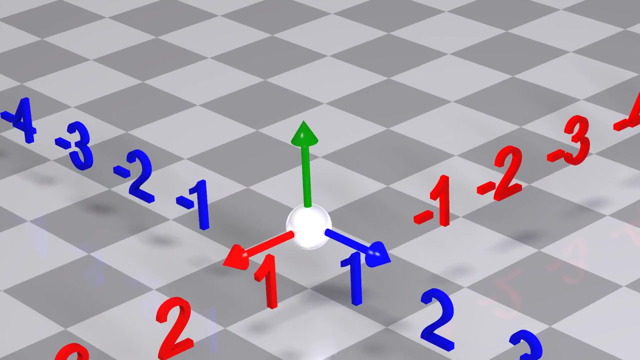 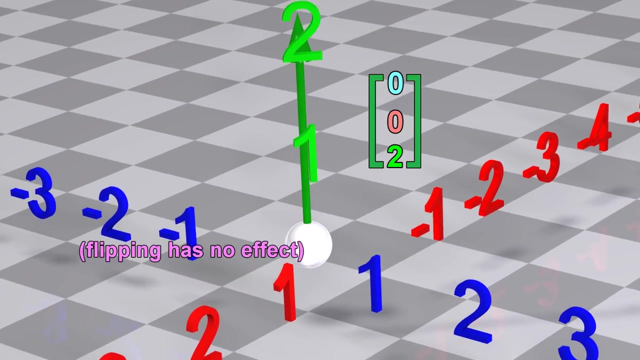 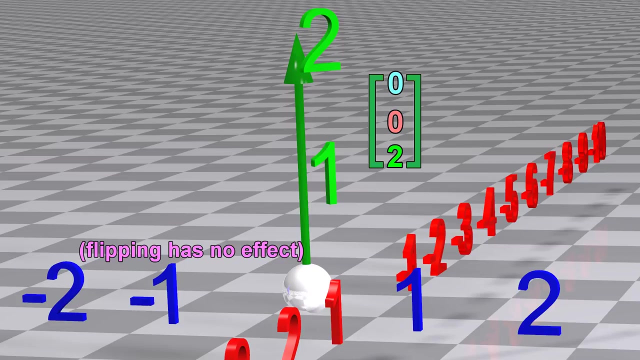 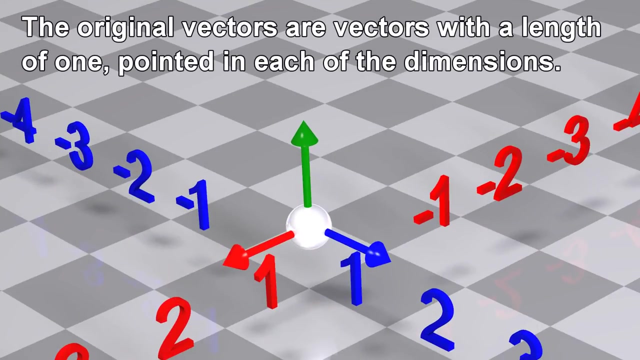 The first is the vector that is to be applied in the linear transformation. The second is the vector that is to be applied in the ring transformation. The third is the vector that is to be applied in the second ring transformation. Thank you, The original vectors are vectors with a length of one. 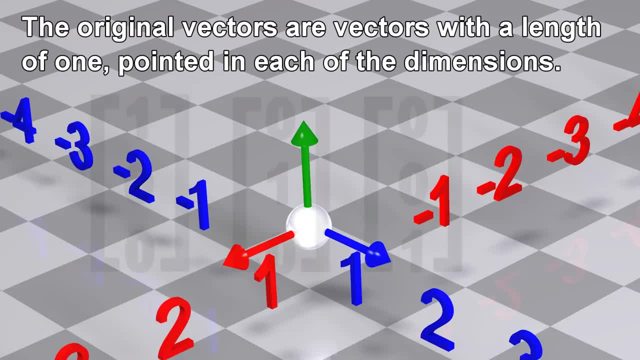 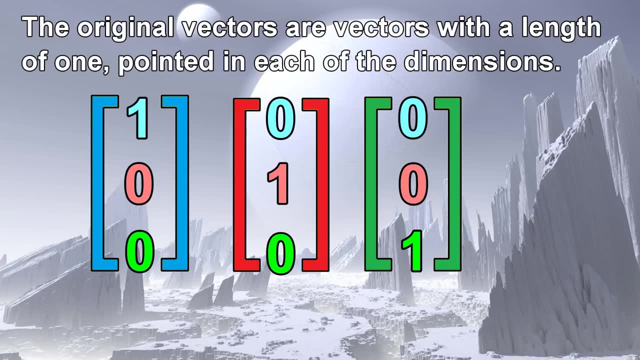 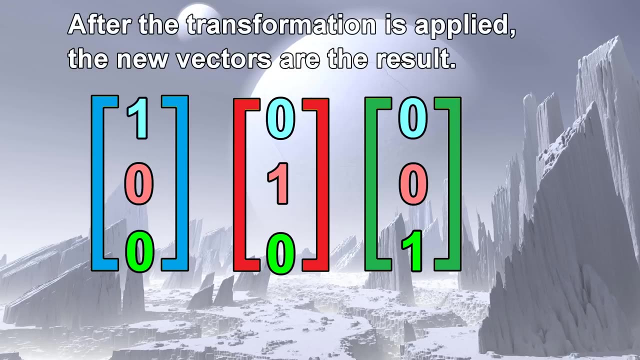 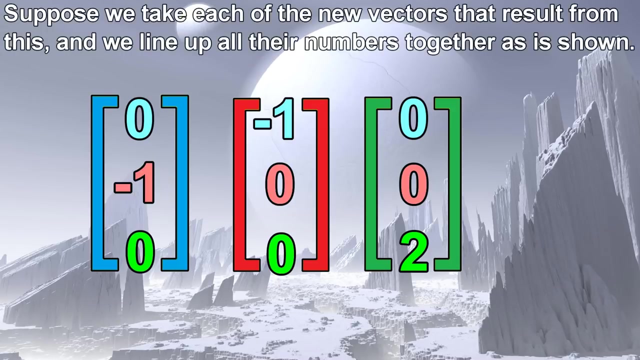 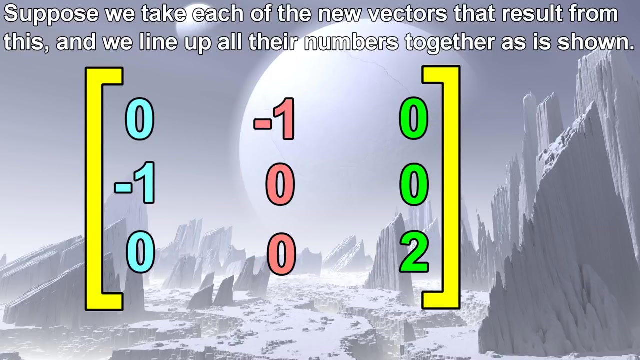 pointed in each of the dimensions. After the transformation is applied, the new vectors are the result. Suppose we take each of the new vectors that result from this and we line up all their numbers together, as is shown, We now have what we call a matrix. 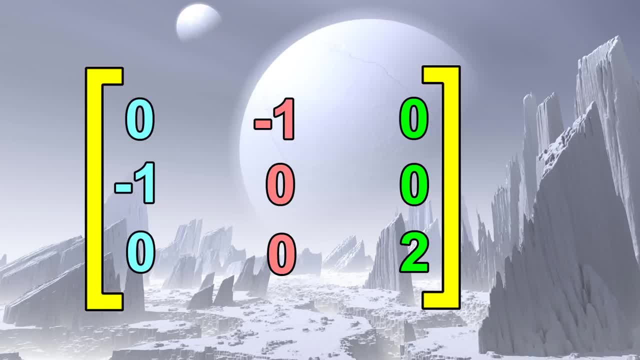 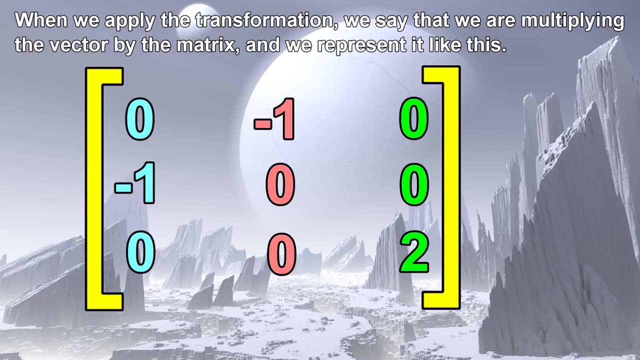 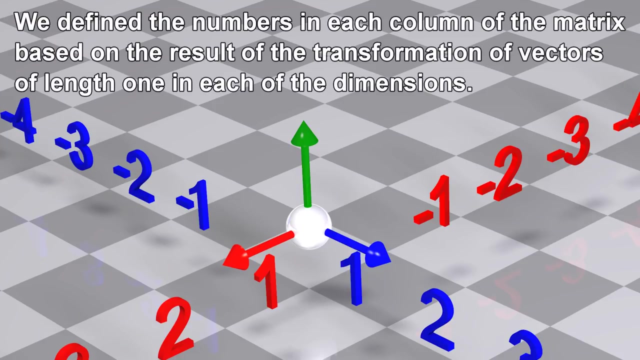 All linear transformations can be represented with a matrix. When we apply the transformation, we say that we are multiplying the vector by the matrix and we represent it like this. We defined the numbers in each column of the matrix based on the result of the transformation of vectors. 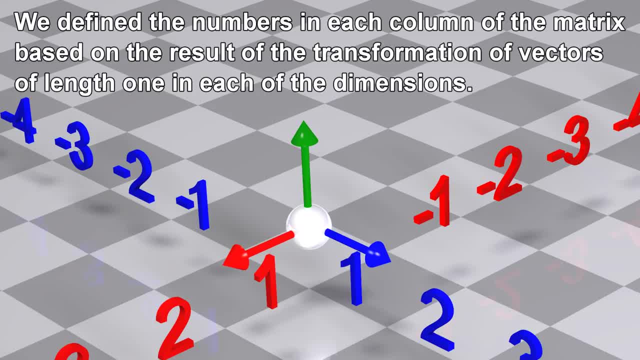 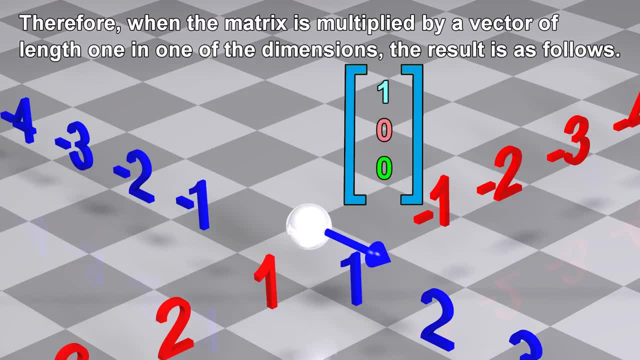 of length, one in each of the dimensions. Therefore, when the matrix is multiplied by a vector of length one in one of the dimensions, the result is as follows: When positive and negative times end, the result is this vector. in this vector, The new vector is the vector participants. 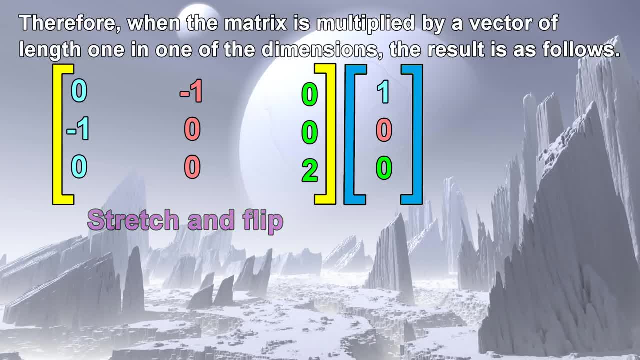 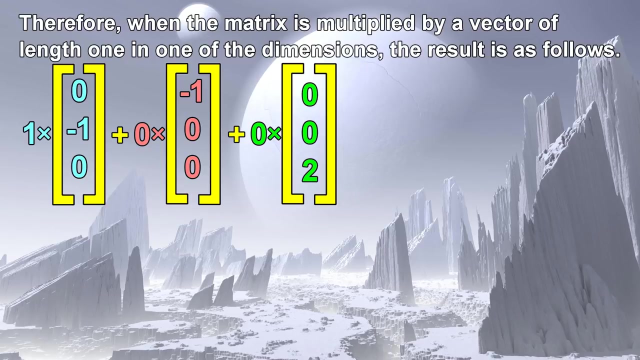 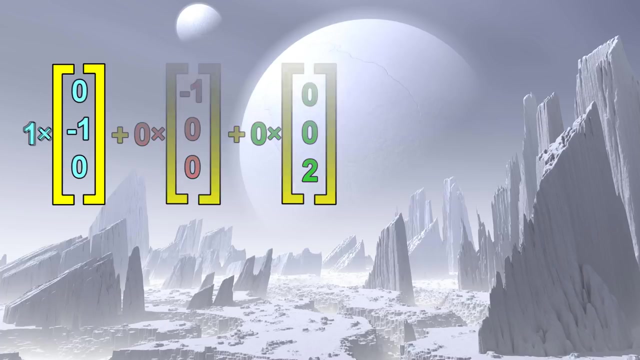 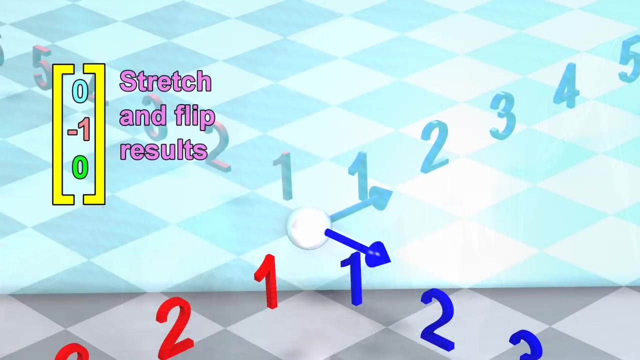 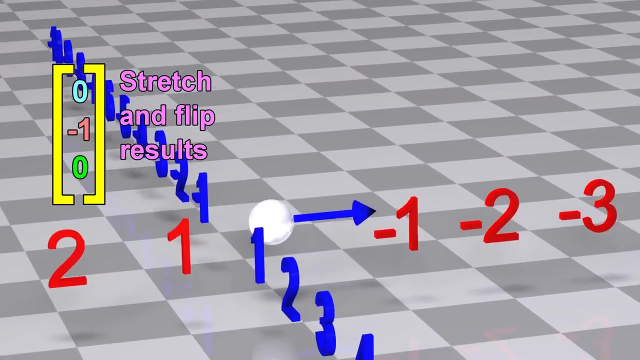 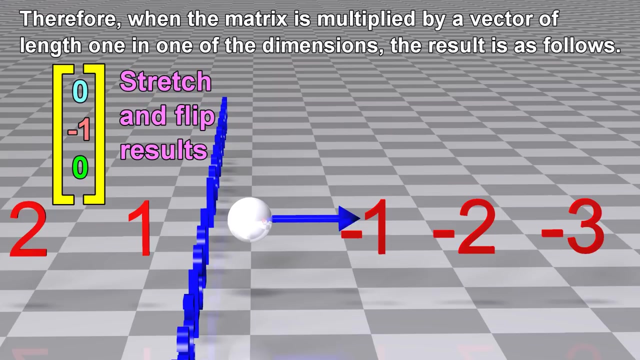 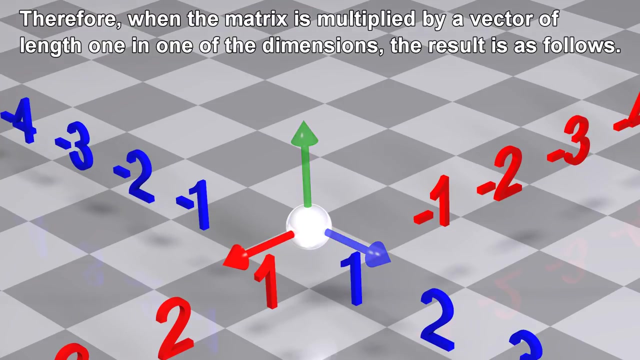 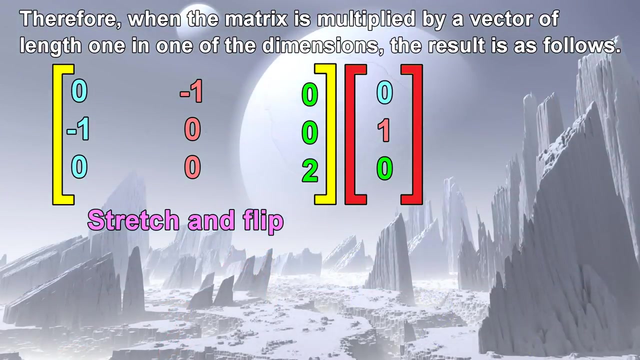 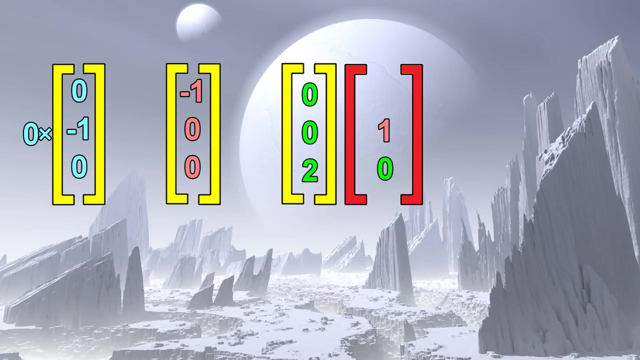 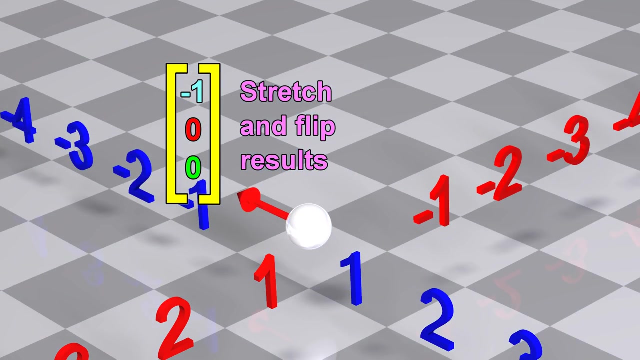 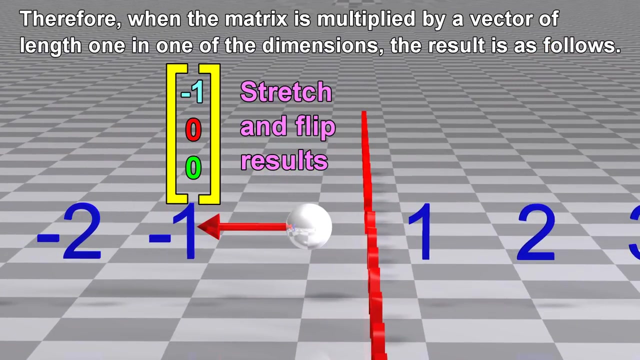 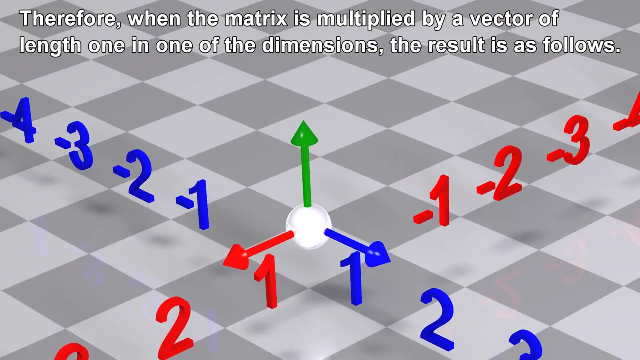 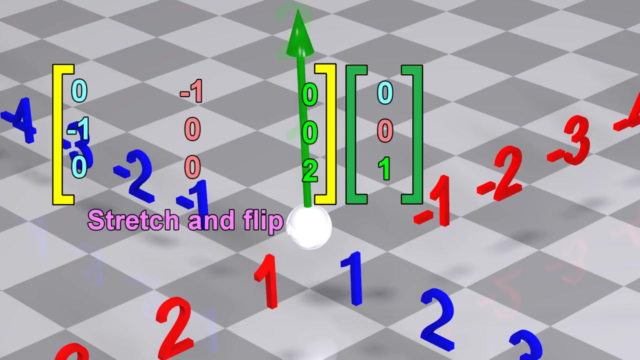 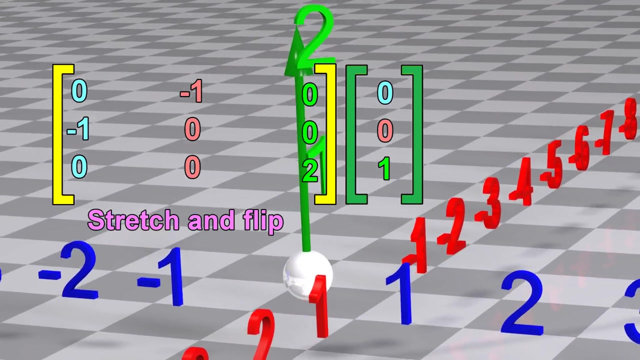 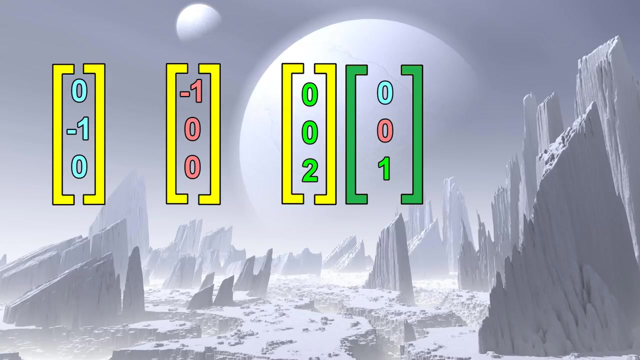 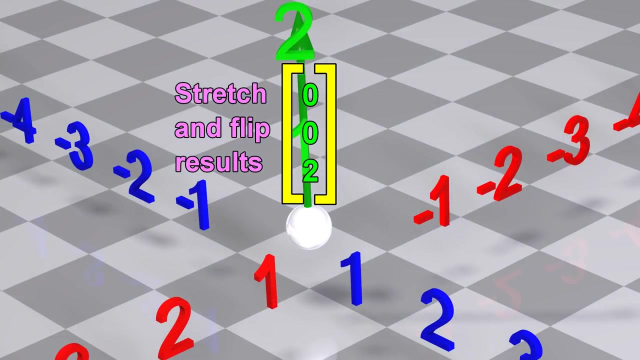 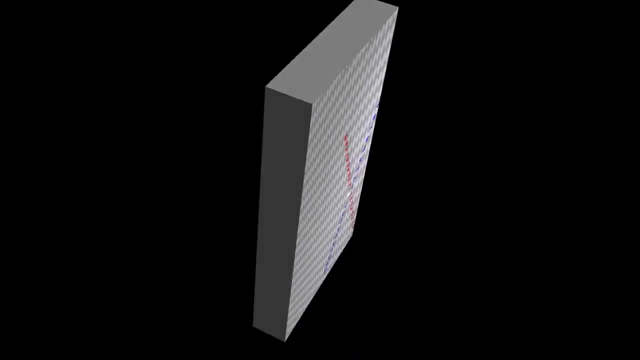 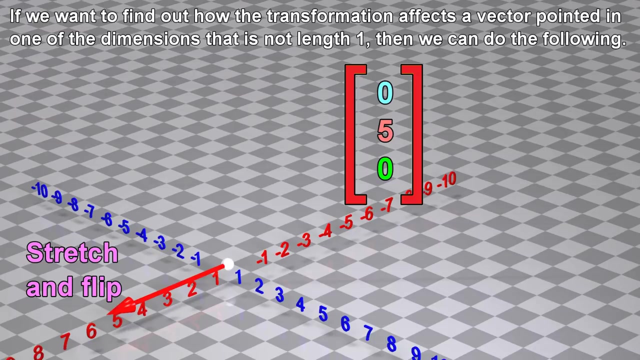 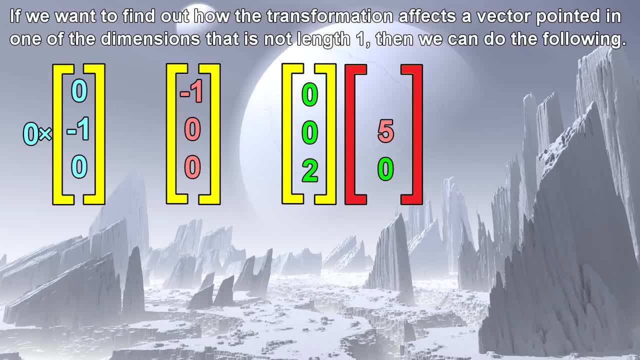 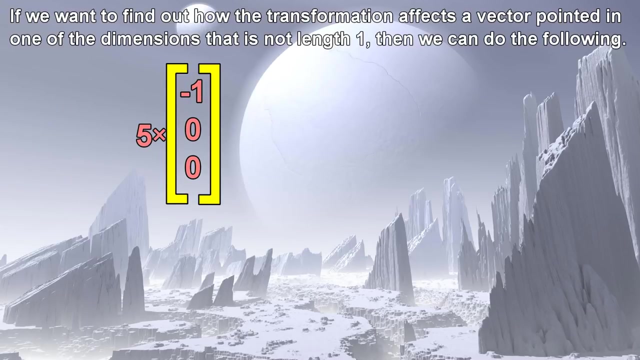 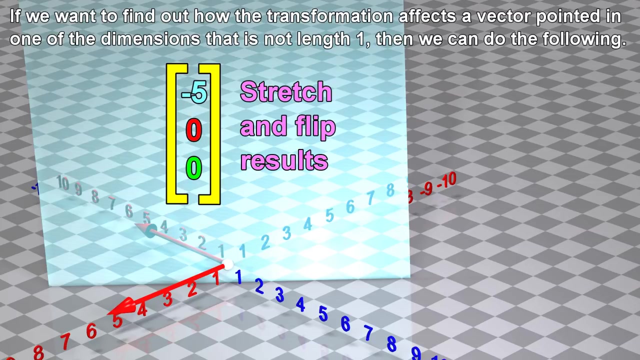 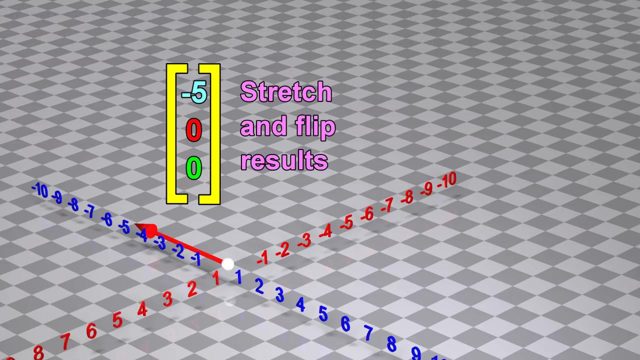 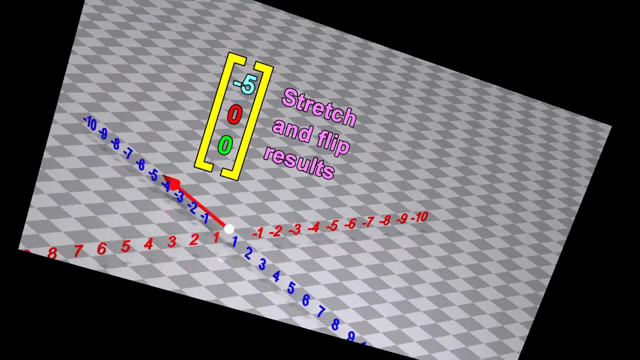 If we want to find out how the transformation affects a vector pointed in one of the dimensions that is not length 1,, then we can do the following. If we want to find out how the transformation affects a vector pointed in one of the dimensions that is not length 1,, then we can do the following. 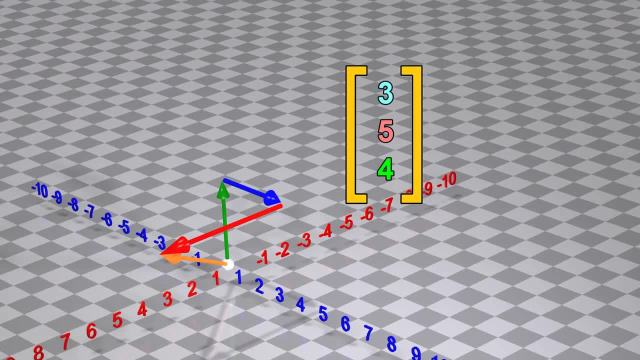 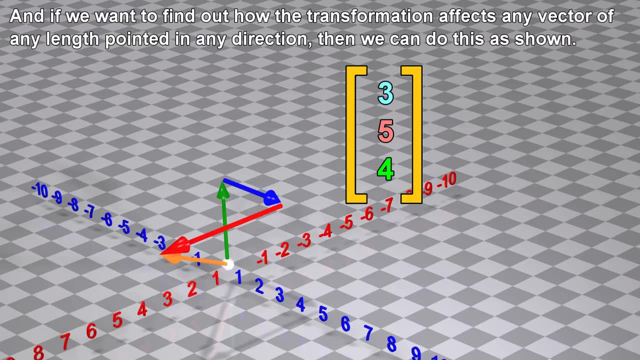 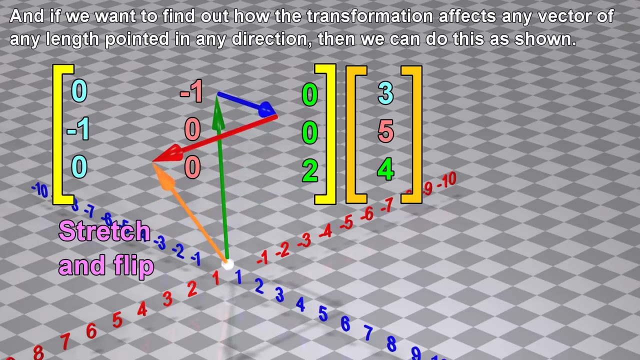 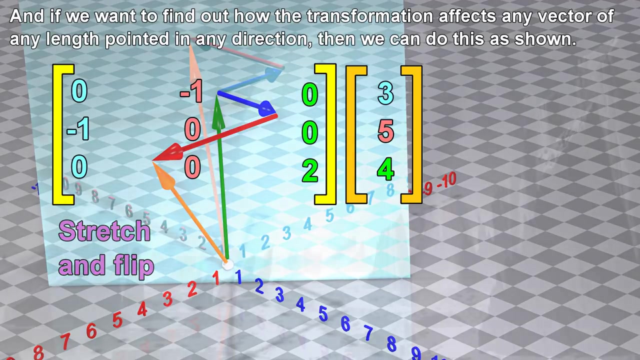 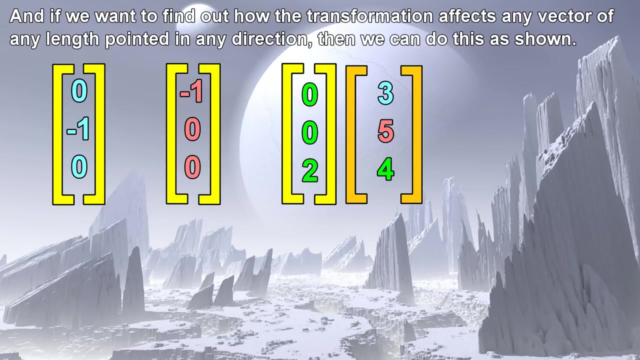 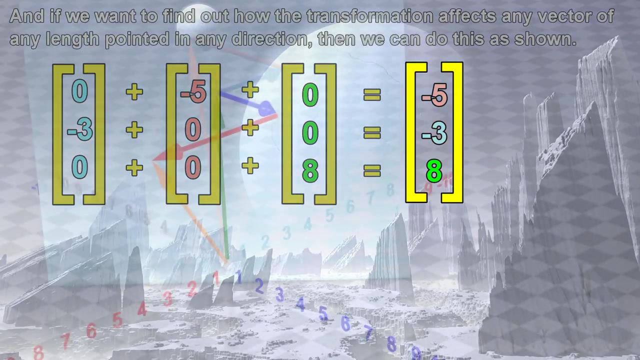 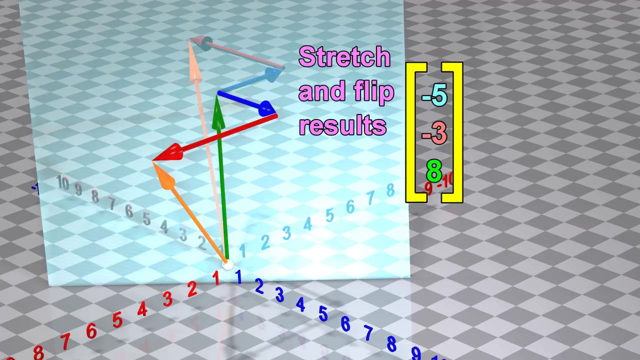 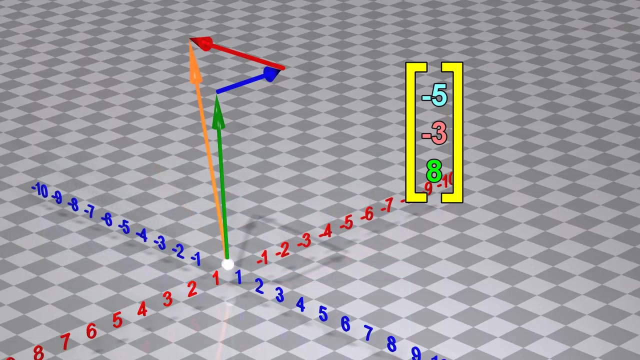 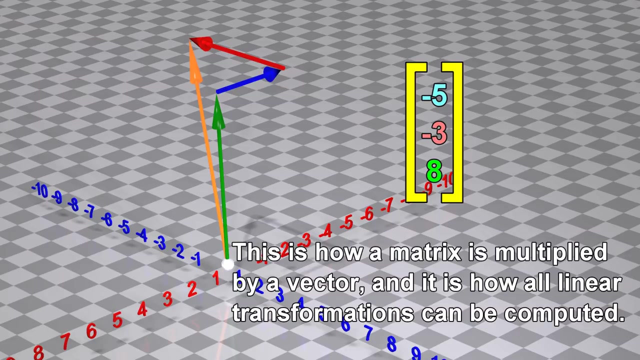 If we want to find out how the transformation affects any vector of any length, pointed in any direction, then we can do this as shown. Thank you, Thank you, Thank you. This is how a matrix is multiplied by a vector and it is how all linear transformations can be computed.